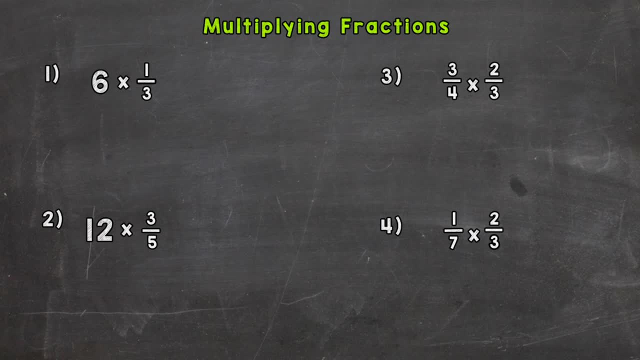 fraction. Now, when we multiply fractions, all we need to do is multiply straight across. So numerator times numerator and denominator times denominator. So the first thing we need to do with this six is make it into a fraction. Whenever you have a whole number, you can. 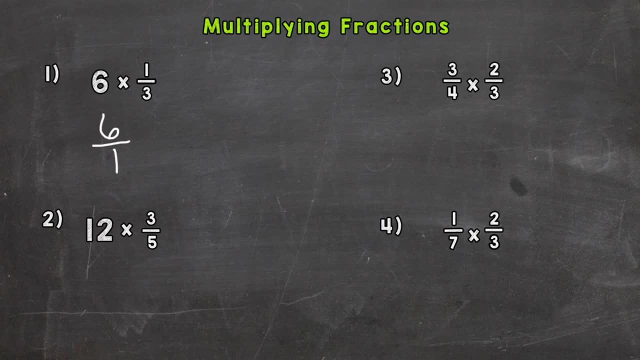 make it into a fraction by putting it over one. That way you have a fraction. You have a numerator and a denominator. Bring down the multiplication sign and the one-third. Now we multiply straight across. Numerator times numerator. Denominator times denominator. 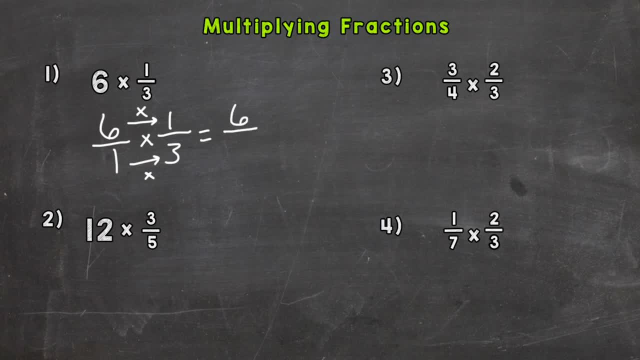 So six times one is six, One times three is three, So our answer is six-thirds. But that's an improper fraction, meaning the numerator, the top number, is lower than the denominator, The bottom number. So you never leave an answer. 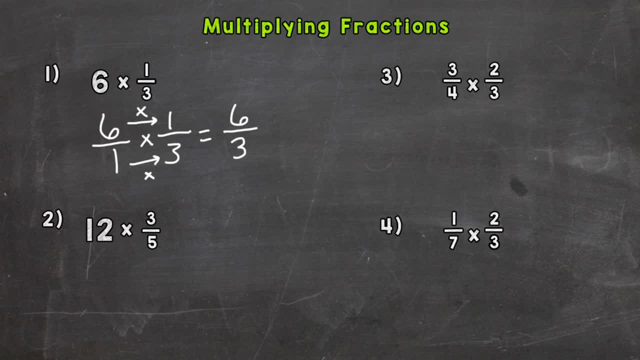 improper. So how to convert it out of improper fraction? we need to divide the numerator, the top number, by the denominator. So six divided by three, That's going to give us a whole number here. So how many whole groups of three can we pull out of six? Well, two. 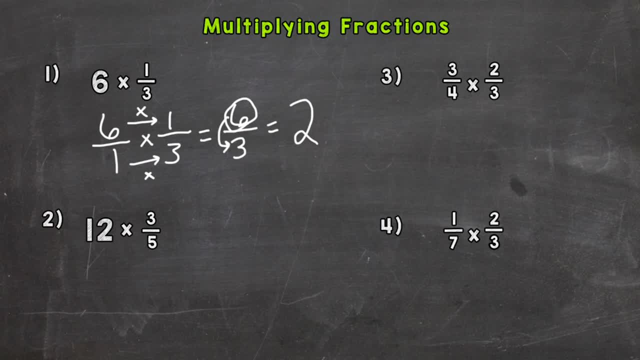 Now, once we do that, is there anything left over remainder? No, So our answer is 2.. So 6 times 1, third is 2.. Now I want you to take a look at this answer compared to our problem, because normally we think 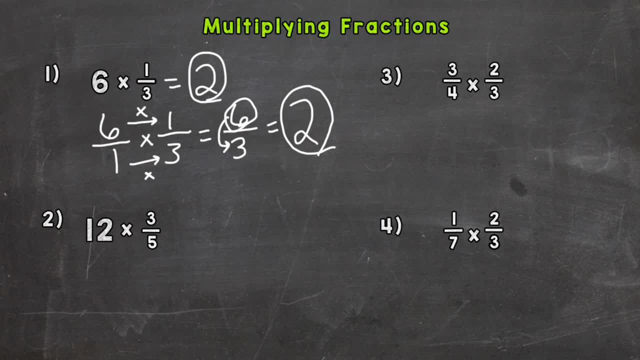 when we multiply two numbers, we should get larger in value. Our answer: should grow in value, right? If you did 6 times 2, we get 12.. But here we started with a 6 and we ended up with a 2. And that's because we multiplied by a fraction. 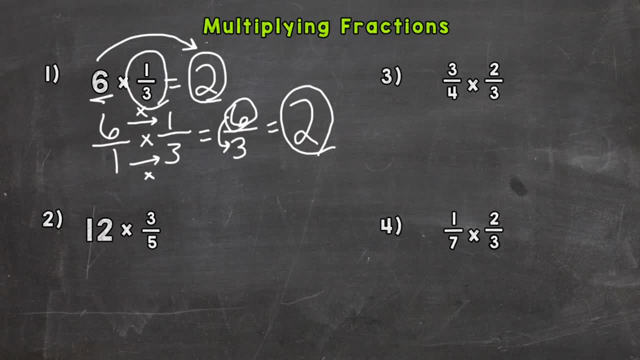 that's less than one whole. So whenever you multiply by something less than a whole, you actually your answer is going to decrease in value from what you started with. So let's take a look at number 2. We have 12. So it's a whole. 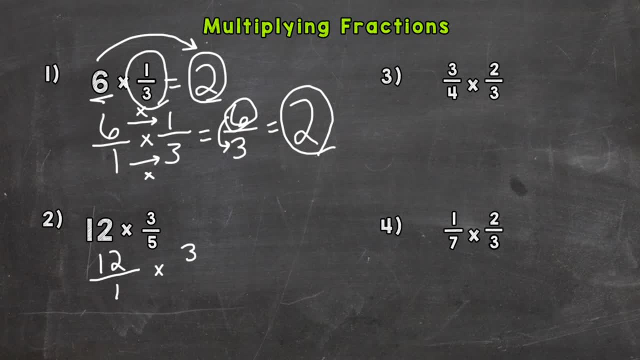 number. Let's put it over 1 and we multiply by 3 fifths, So go straight across 12 times 3.. 36. 1 times 5 is 5.. So 36 fifths. So what we need to do now? that's our answer. but 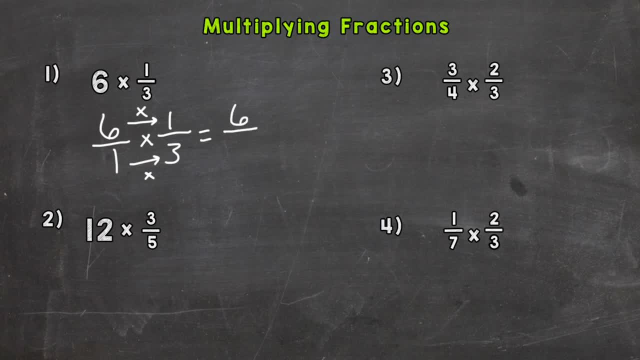 So six times one is six, One times three is three, So our answer is six-thirds. But that's an improper fraction, meaning the numerator, the top number, is lower than the denominator, So you never leave an answer improper. So how to convert it out of improper fraction? 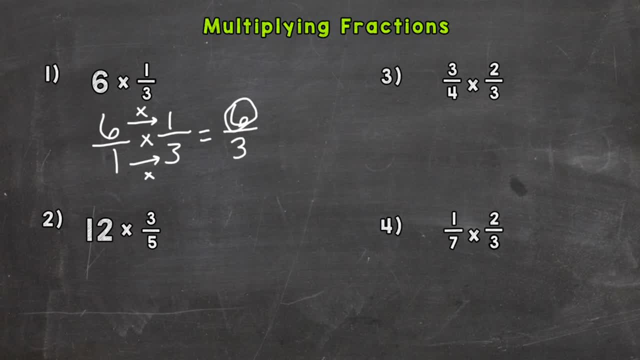 we need to divide the numerator, the top number, by the denominator. So six divided by three, That's going to give us a whole number here. So how many whole groups of three can we pull out of six? Well, two Now. once we do that, is there anything left over? Is there a whole? 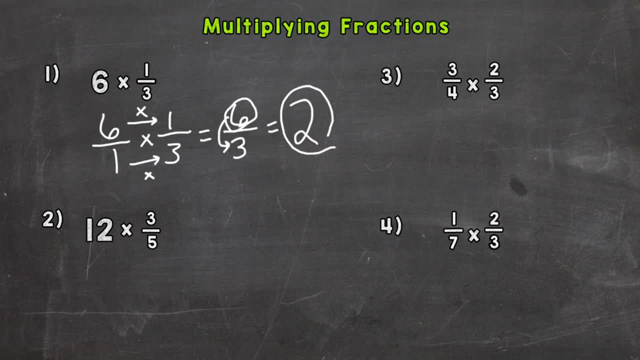 remainder No. So our answer is 2.. So 6 times 1, third is 2.. Now I want you to take a look at this answer compared to our problem, because normally we think when we multiply two numbers we should get larger in value. Our answer should: 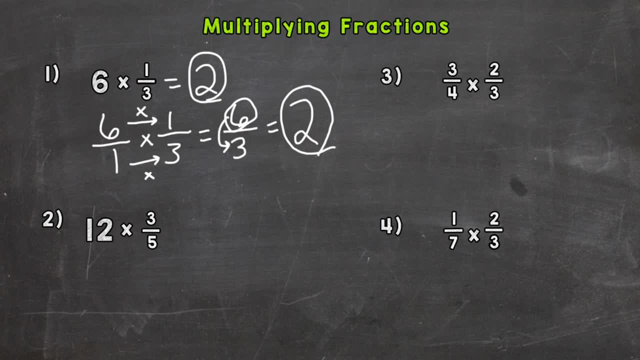 grow in value. right, If you did 6 times 2, we get 12.. But here we started with a 6 and we ended up with a 2. And that's because we multiplied by a fraction that's less than one whole. So whenever you multiply by something less than a, 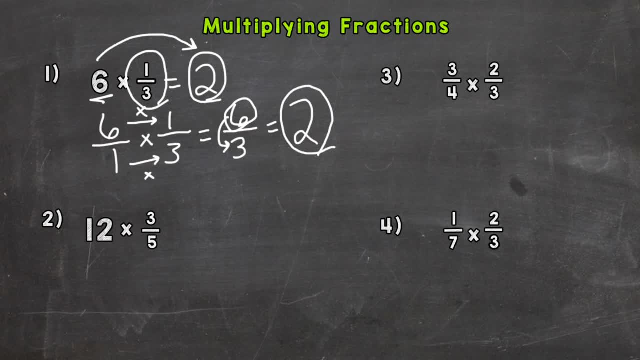 whole you actually your answer is going to decrease in value from what you started with. So let's take a look at number 2.. We have 12. So it's a whole number. Let's put it over 1 and we multiply by 3 fifths, So go straight. 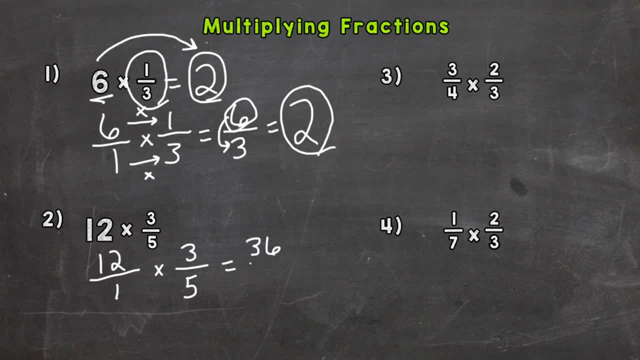 across 12 times 3.. 36.. 1 times 5 is 5.. So 36 fifths. So what we need to do now? that's our answer, but it's improper. So we need to divide the numerator by the denominator, So 36. 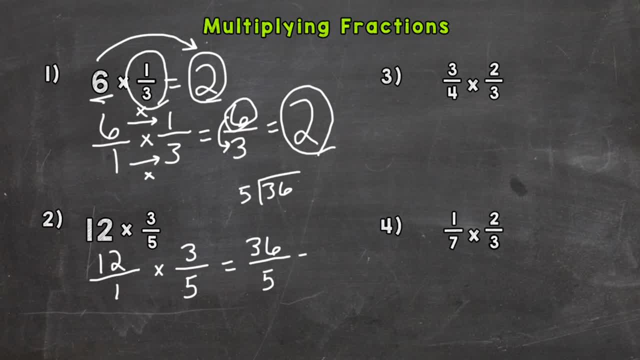 divided by 5.. So how many whole groups of 5 can we pull out of 36?? And the answer is 7 wholes. So that's our whole number here, But we didn't hit 36 exactly. We have a remainder or something left over, So 7. 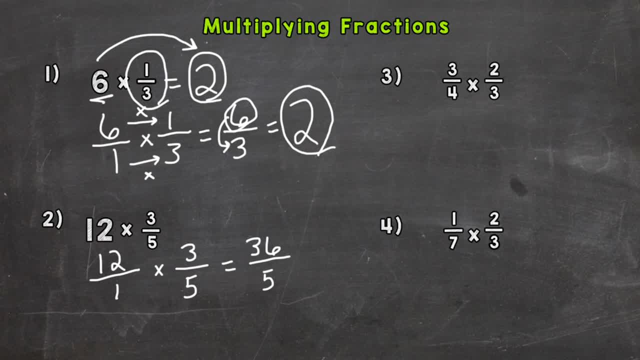 it's improper. So we need to divide the numerator by the denominator, So 36 divided by 5.. So how many whole groups of 5 can we pull out of 36?? And the answer is 7 wholes. So that's our whole number here. 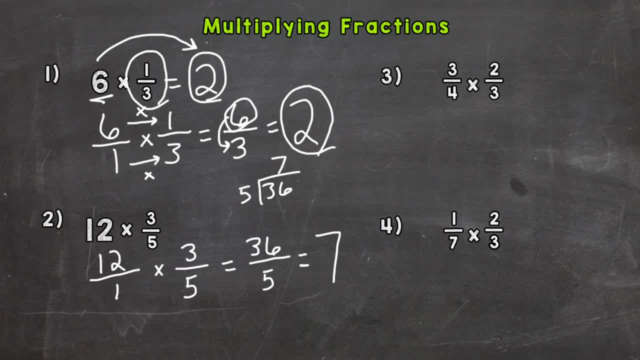 But we didn't hit 36 exactly. We have a remainder or something left over. So 7 times 5 is 35.. Subtract to find out what the remainder is, And it's 1.. So that 1 is actually going to be the numerator of our fractional part of this mixed number. 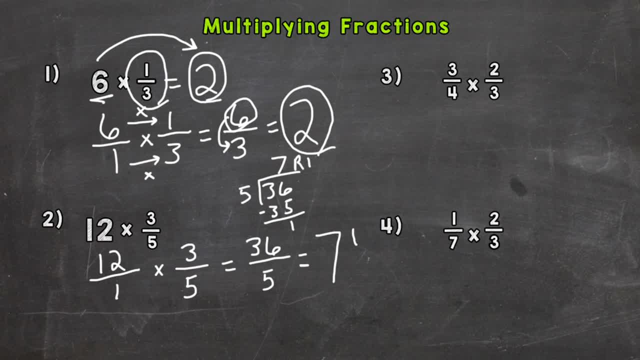 A mixed number has a whole number and a fraction, So our remainder is the numerator And we keep the denominator the same. So we bring that 5 over, So 7 and 1 fifth. So again we started with 12 and we multiplied by something. 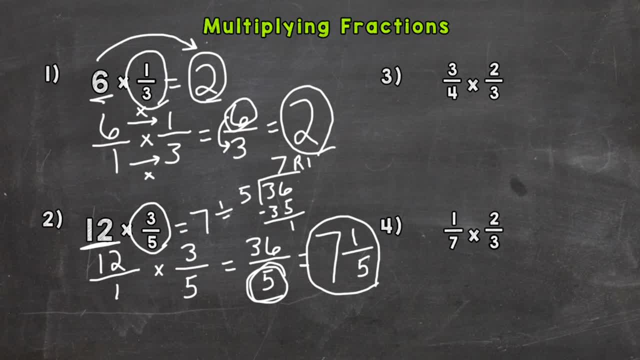 less than a whole. So our answer actually decreased in value relative to what we started with in the problem, And that's okay because we multiplied by something less than one whole. So number 3, we have 3 fourths times 2.. 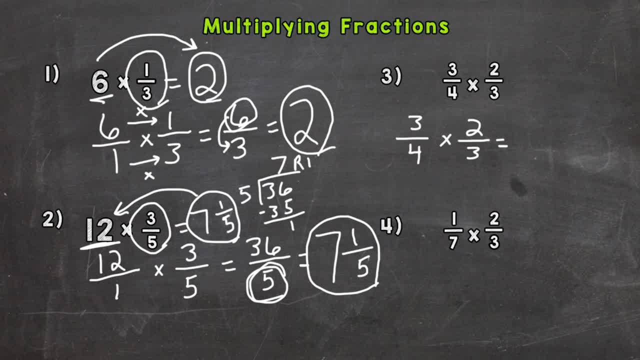 Alright, straight across, 3 times 2 is 6, and 4 times 3 is 12.. So our answer is 6 twelfths. Now that fraction can be simplified. It's a proper fraction, but we have a greatest common factor between the 6 and the 12: that 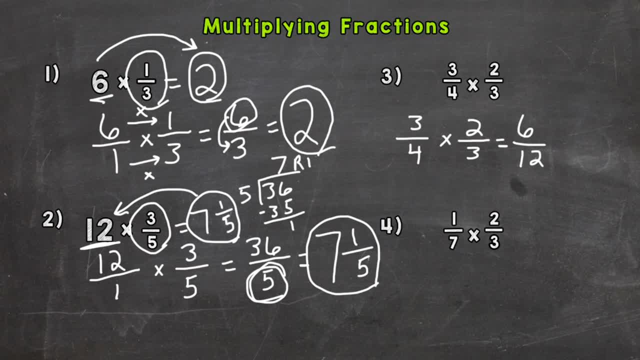 we can break down or simplify this fraction into its lowest terms, And that greatest common factor is 6.. So let's divide both of these by 6.. 6 divided by 6 is 1, and 12 divided by 6 is 2.. 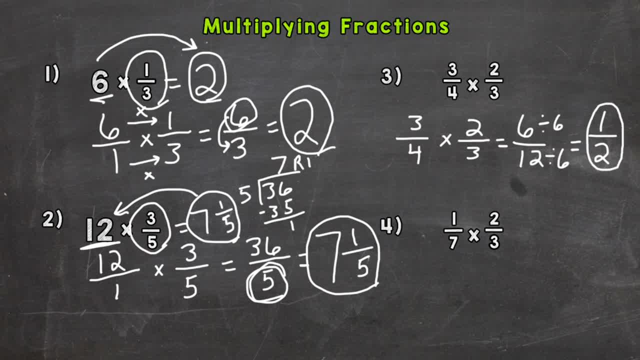 Now that fraction cannot be broken down anymore. The only common factor between 1 and 2 is 1, so we are done. The answer to number 3 is 1, half Alright. number 4, we have 1 seventh times 2 thirds. 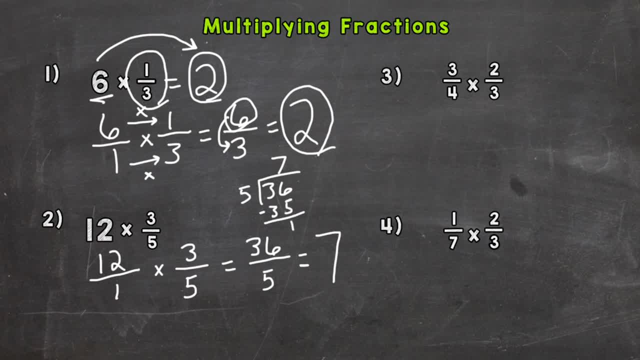 times 5 is 35.. Subtract to find out what the remainder is, And it's 1.. So that 1 is actually going to be the numerator of our fractional part of this mixed number. A mixed number has a whole number and a fraction, So our remainder is the. 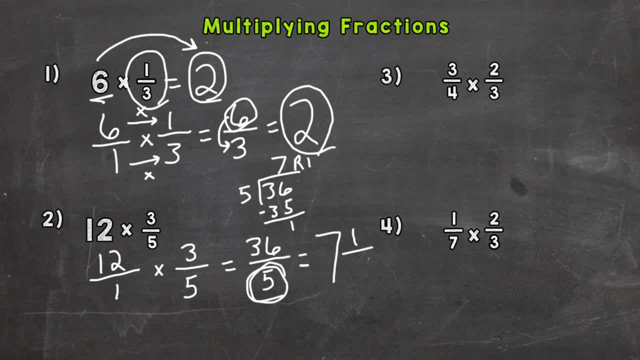 numerator And we keep the denominator the same. So we bring that 5 over, So 7 and 1 fifth. So again we started with 12 and we multiplied by something less than a whole. So our answer actually decreased in value relative to what we started with. 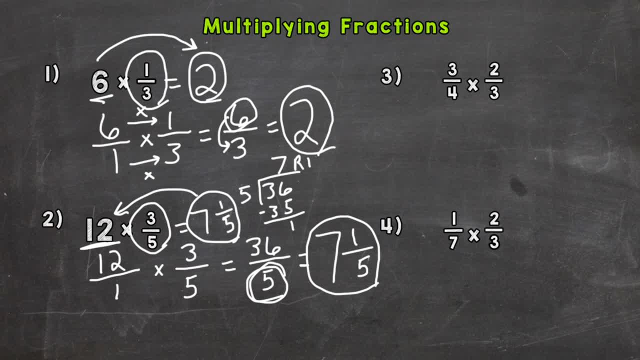 in the problem, And that's okay, because we multiplied by something less than one whole, So number 3, we have 3 fourths times 2.. Thirds, Alright, straight across: 3 times 2 is 6. And 4 times 3 is 12.. So our answer: 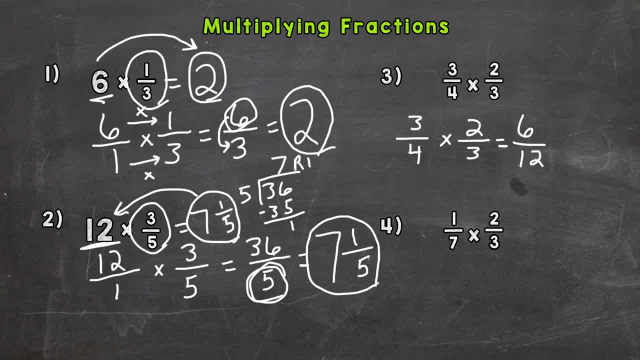 is 6 twelfths. Now that fraction can be simplified, It's a proper fraction, but we have a greatest common factor between the 6 and the 12: that we can break down or simplify this fraction into its lowest terms, And that greatest common factor is 6.. 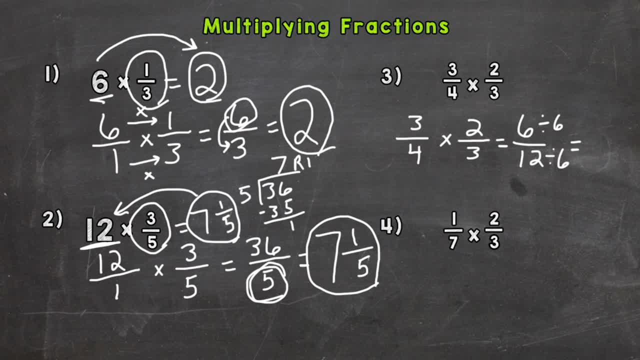 So let's divide both of these by 6.. 6 divided by 6 is 1. And 12 divided by 6 is 2.. Now that fraction cannot be broken down anymore. The only common factor between 1 and 2 is: 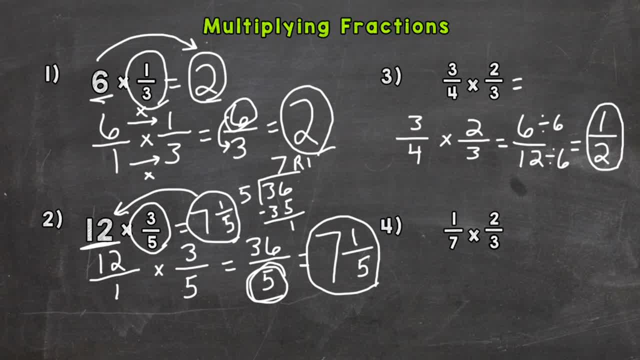 1.. So we are done. The answer to number 3 is 1, half Alright. number 4, we have 1, seventh times 2, thirds Straight across. 1 times 2 is 2. And 7 times 3 is 21.. 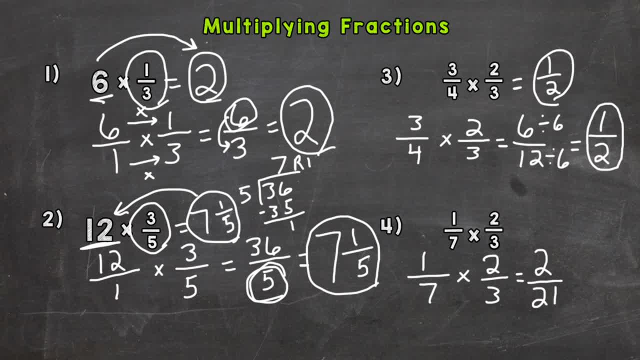 So we get 2 over 21.. Now the only common factor between 2 and 21 is 1. So we are simplified here. That's as far as that fraction can break down. So we are done: 2 over 21..